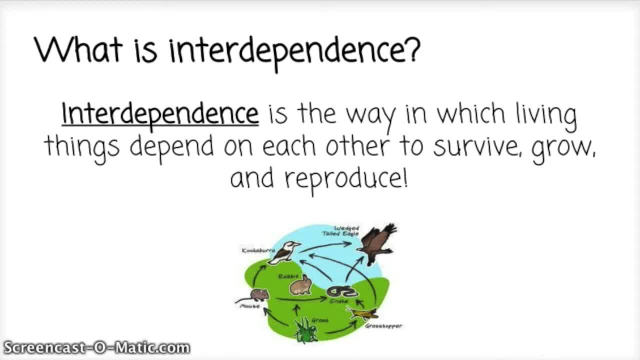 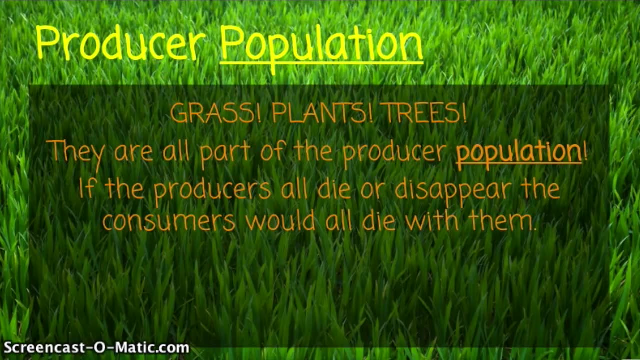 For example, the grasshopper needs the grass to eat and to survive, and then, next, the snake depends on the grasshopper to eat and the eagle will eat the snake. What would happen if there was disruption in the food chain? Well, first we need to know the two types of populations. First is the producer population. These are living organisms that make their own food, For example, grass, plants and trees. 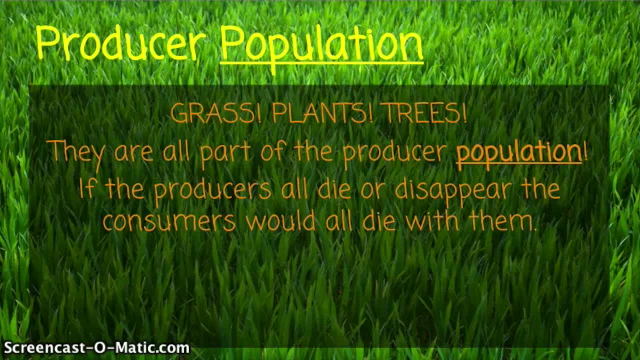 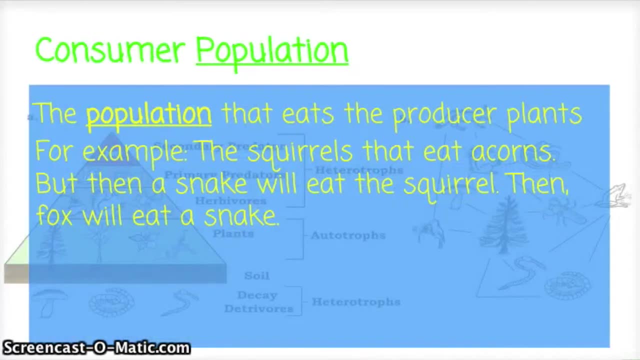 If the producers all die or disappear, the consumers, or the consumer population, would all die with them. The consumer population: This population is the population that eats, the producer population. For example, the squirrel eats acorns and that acorn would be considered as a producer population. 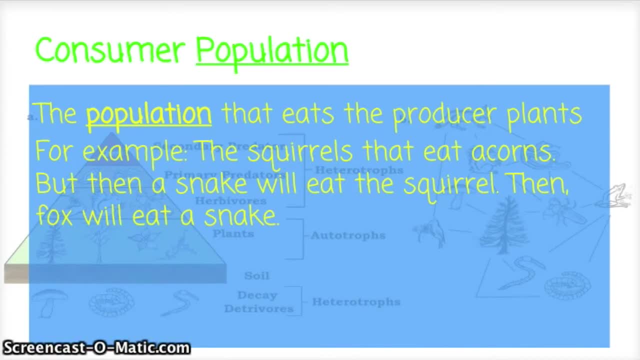 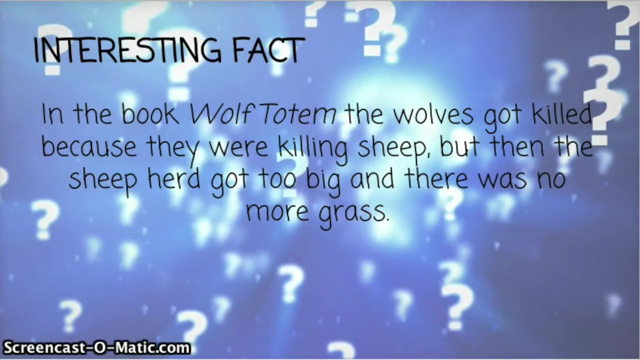 And then next, the snake will eat the squirrel, and the snake would be the consumer, and the squirrel would be the consumer, And then a fox will eat a snake, Which makes the fox a consumer population too. There's a book called Wolf Totem, which is about these people in Mongolia, China, which are basically farmers, and they basically have the same effect of the disruptions. 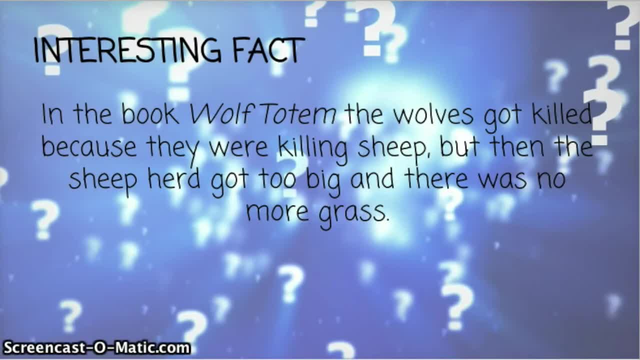 So first what happens is they thought the wolves were killing too much of their sheep, So they kill all the wolves. But then there's no more sheep to kill. so all the sheep, their numbers are doubled. So all the sheep—their numbers are doubled. 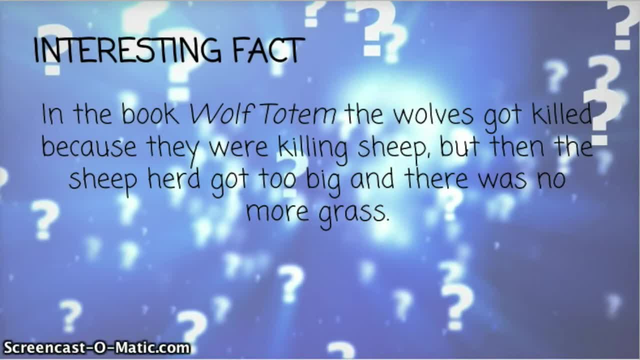 So all the sheep, their numbers are doubled. So all the sheep, their numbers are doubled. So all the sheep, their numbers are doubled. get too big and then they eat too much of the grass and all their grass dies, and that's what. 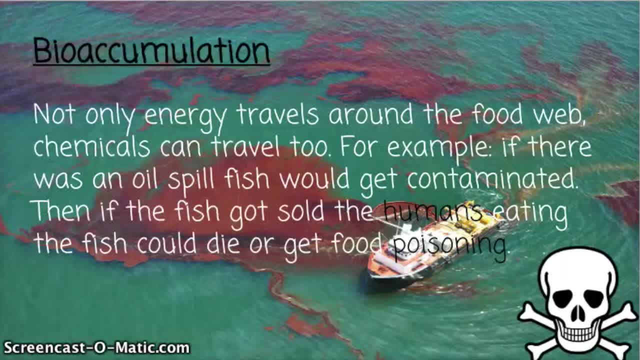 caused a lot of problems in that book. What is bioaccumulation? Bioaccumulation is when chemicals or harmful gases get passed around the food web. For example, when there was an oil spill, fish would get contaminated with all the dirty chemicals. and if these fish got sold to humans? 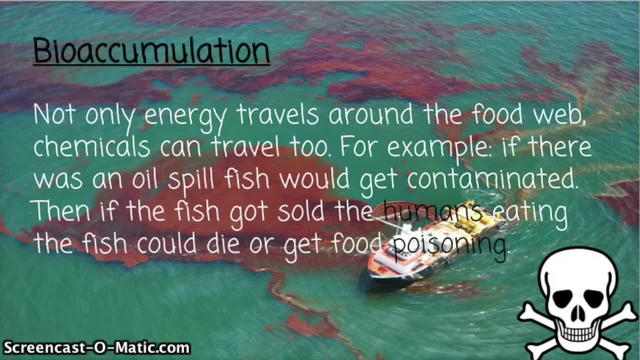 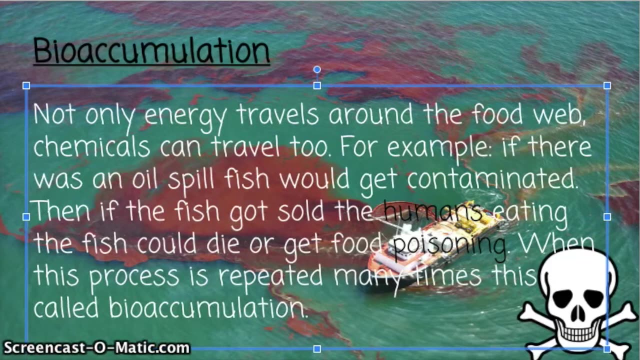 and the humans ate the fish. they could have got food poisoning or some kind of disease, or they can die. This can also happen through normal wild creatures. Bioaccumulation Now. bioaccumulation is a process of when chemical gases or liquids get built up over time and kills the animal.